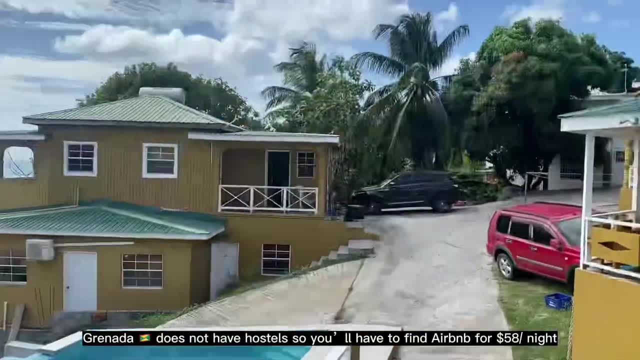 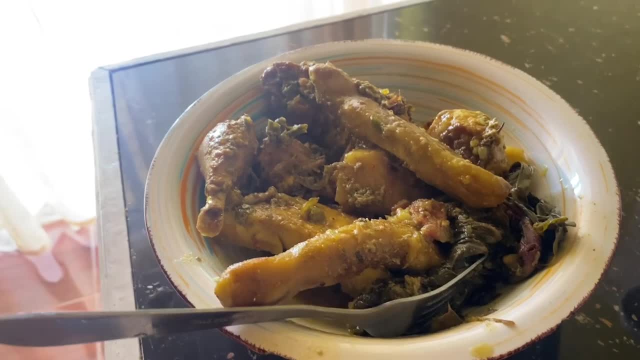 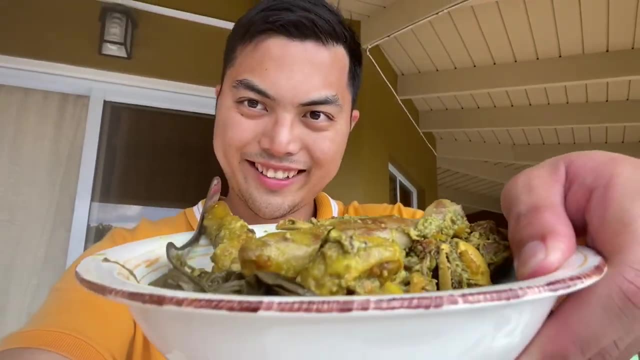 Bradford From that place. Oh, it looks good. It tastes good too. It tastes good too. Yeah, I'll give it a try. Okay, so I'm here in Grenada about to try Oil down. So you have nutmeg on that. 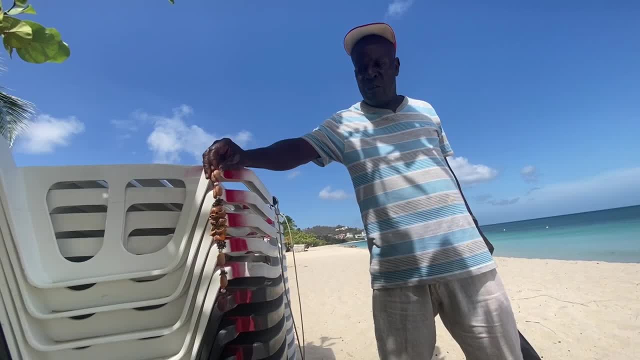 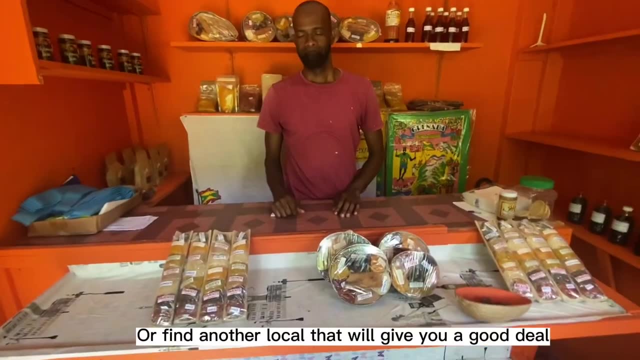 Nutmeg, clove, bay leaf, cinnamon, cocoa beans, ginger, Ginger, Saffron. Okay, Better price than that. How much is a better price? 20?. You get a lot of tourists, Yeah, Okay. So introduce me to your spices. 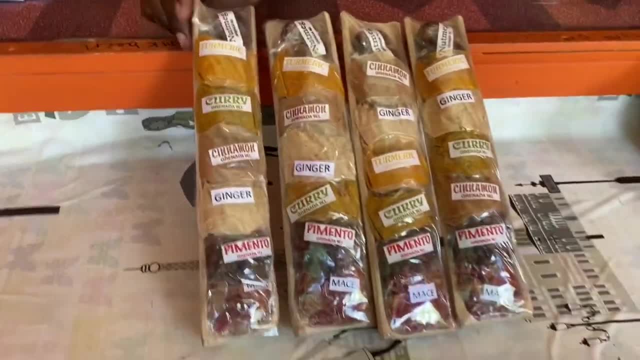 So we have here this is the bamboo- All the different spices. Yeah, Over here this is the calabash, also with the spices. Okay, So over here we got the nutmeg jam, nutmeg jelly, nutmeg syrup. 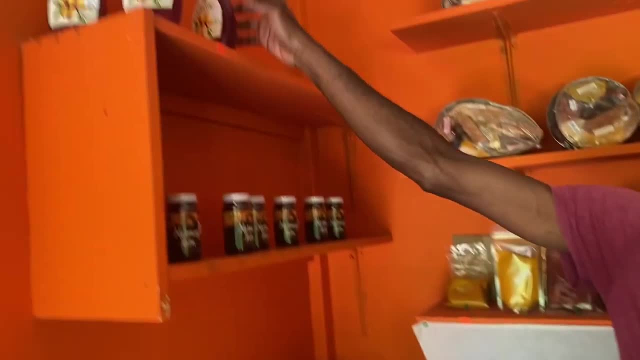 Yeah, All these making the outside part of the nutmeg also as well, Okay. So over here we got all the separate spices- Okay, Different packages. We got the pure honey, Okay. And then that's the chocolate balls where you can make your cocoa tea. 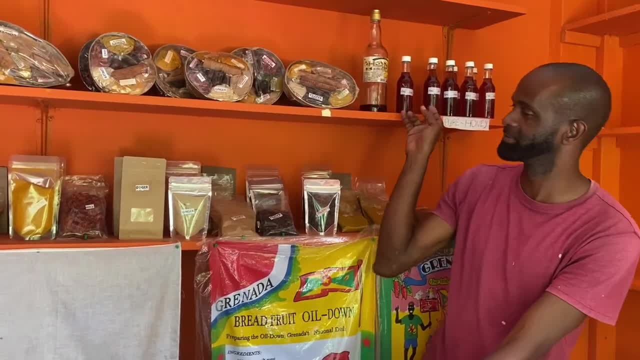 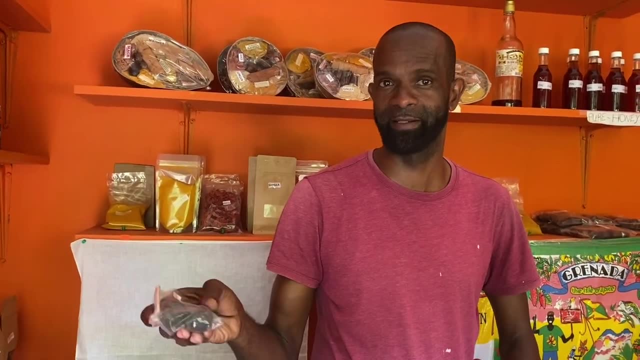 Okay. So you drop one cocoa ball into 35 cups of water. Yeah, You let it boil, Okay, And then you let it cool, Okay, And then you let it cool, Okay, And then you let it cool Okay. 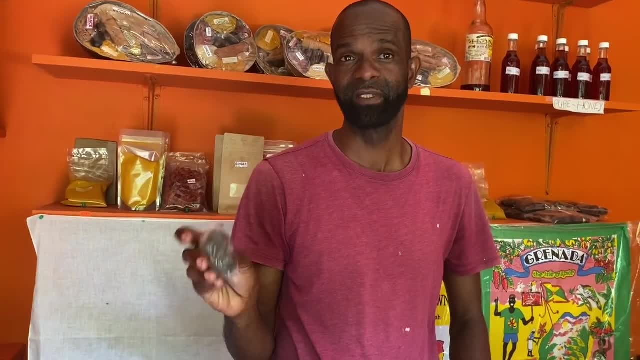 You let it cool, Okay. And then you put the chocolate balls into 35 cups of water- Yeah, You let it boil for at least five minutes. The whole thing would dissolve. When it's dissolved, you add your milk and your sugar and you make a nice cup of hot. 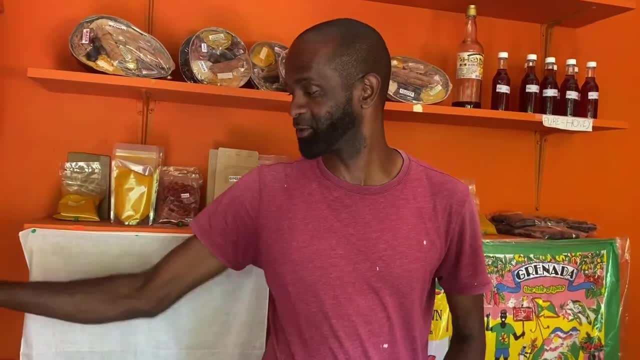 chocolate. Oh, in green it says cocoa tea, And also that's the sauce as well. Cocoa balls- Okay, Cocoa balls, And I made it myself. Oh, you made it all for yourself, Okay, So here we have your recipe. 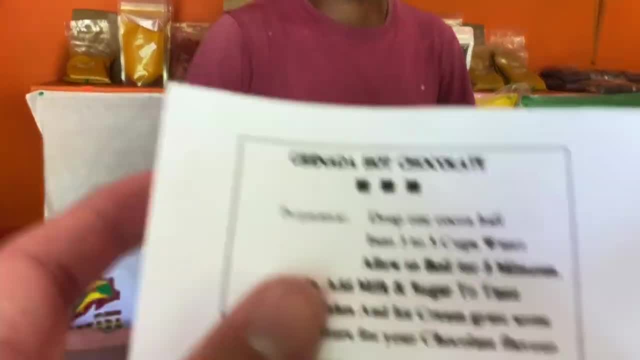 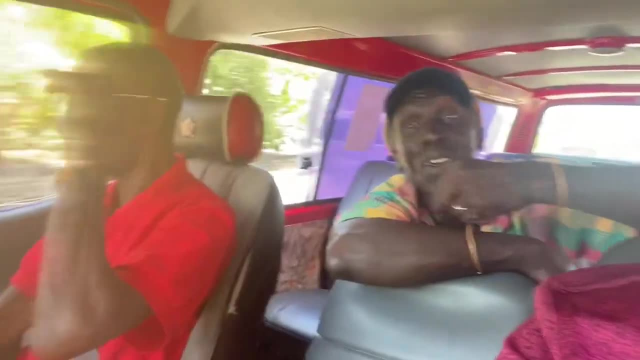 Yeah, This is how to make the hot chocolate. Okay, Interesting. Come on, Grenada, Let's go, Let's go. Come on Grenada. Come on Grenada, Come a Grenada. we love you all the while. 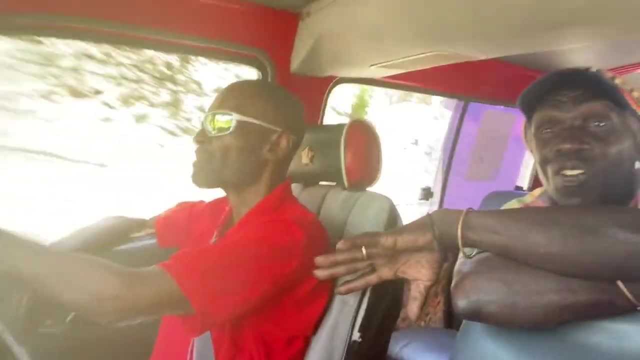 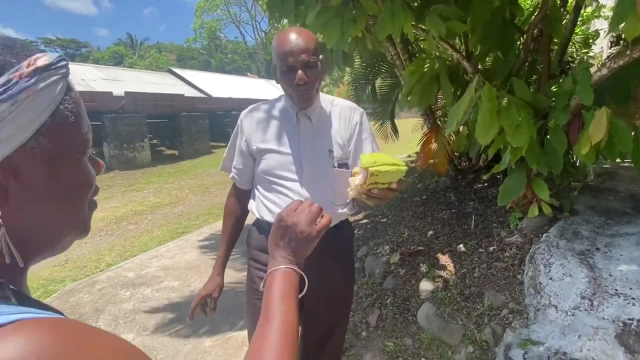 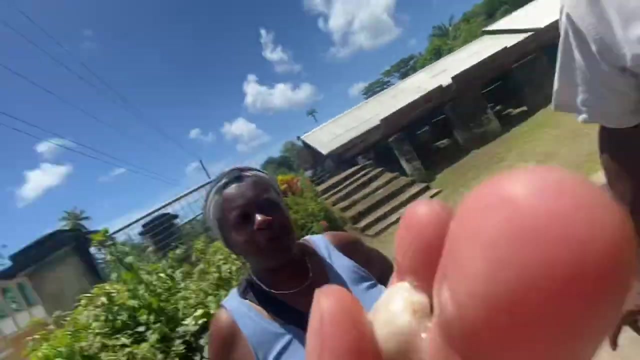 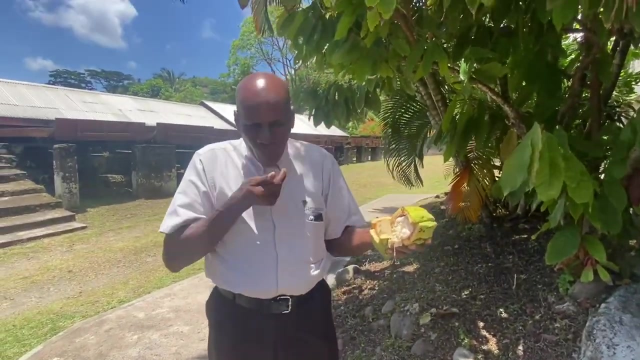 My driver is Bupa. Us face on the scene. well, well, clean When we come a Grenada, Oh nice, right up here, Wonderful, Don't bite it, just suck it. The raw cocoa is on the inside. Okay, Now it goes through that process. 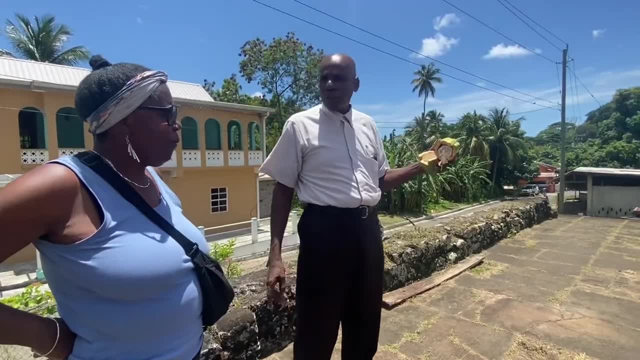 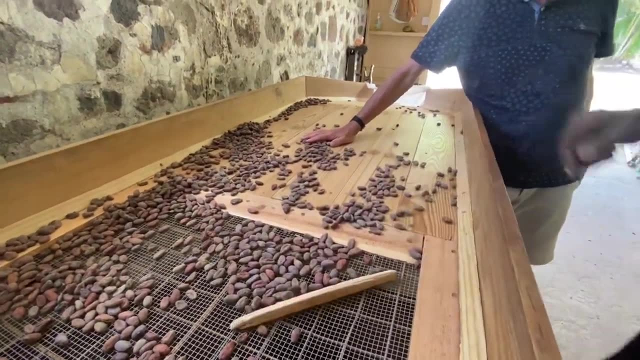 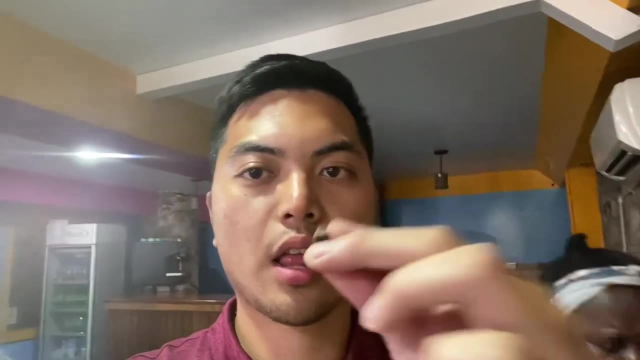 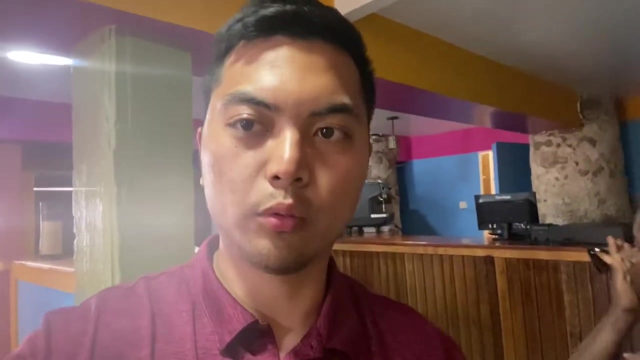 So process number one, the fermentation stage. Well, this is what we use eventually after: Okay, So you suck it out here, You put it in the bag. That one's a little rough. Oh, you can smell it from here. 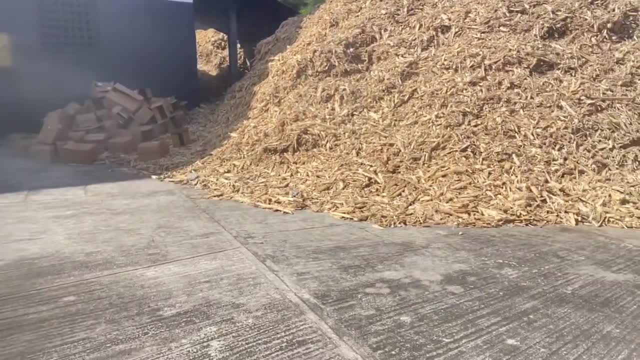 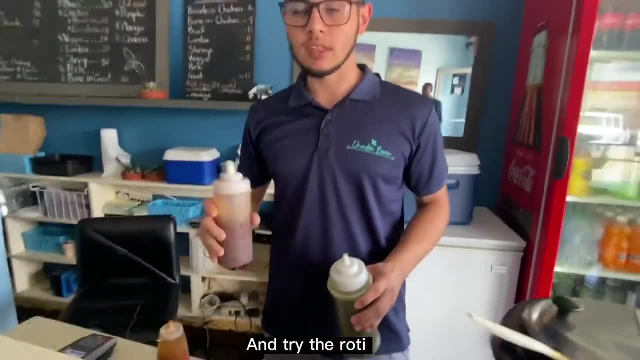 Is there any smoke coming from? So what's this one? This is called Tamarind- Tamarind, It's more like a sweet sauce. And what's that one? This is Chardonnay and it's kind of like cilantro, but it's a lot stronger. 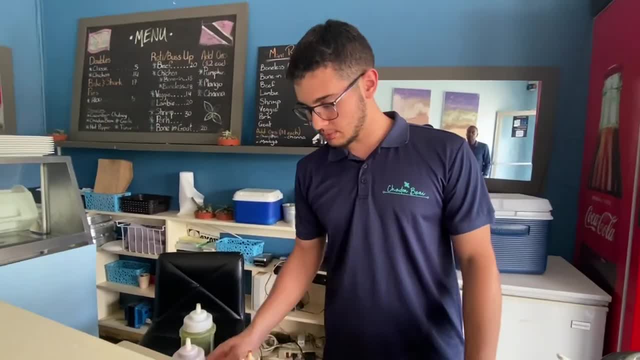 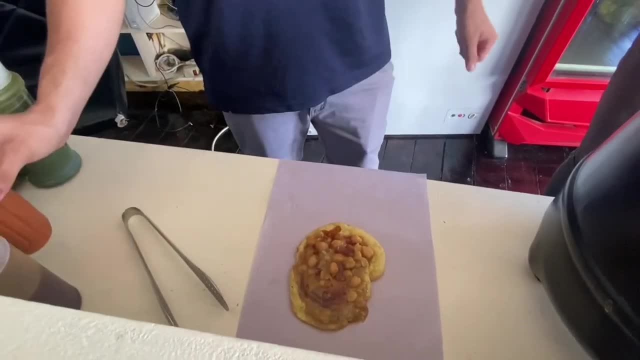 Oh, okay, I think I'll get the sweet one. Sweet Yeah, Okay, Any hot sauce? Oh no, You know, you should try a little bit of the Chardonnay. Chardonnay, I think the Chardonnay is the double. 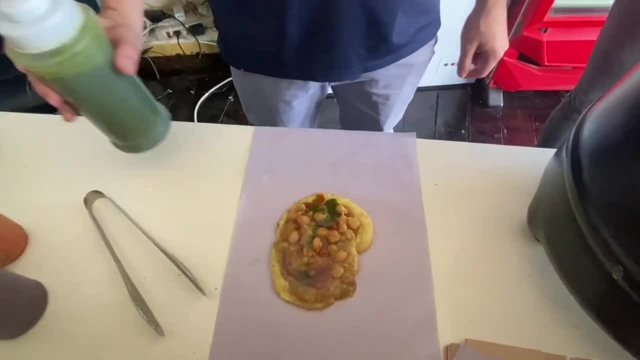 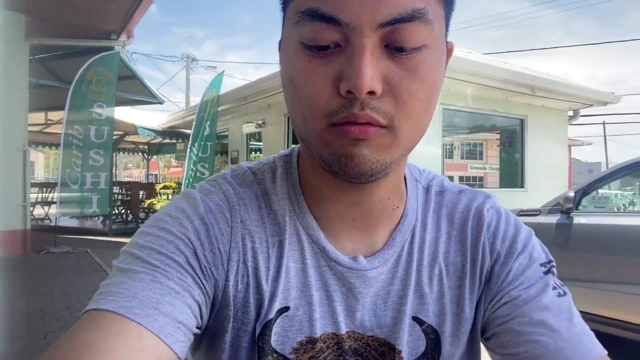 Just a little bit, All right. Yeah, Just for the. I think that was kind of small amount. That's good, All right, Thank you, You're welcome, And that's. I'm here in Grenada about to try the roti and the doubles. 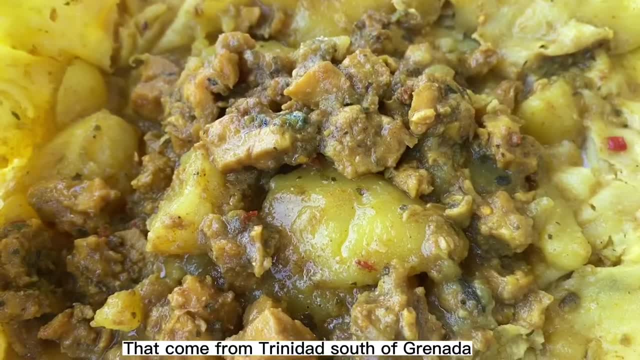 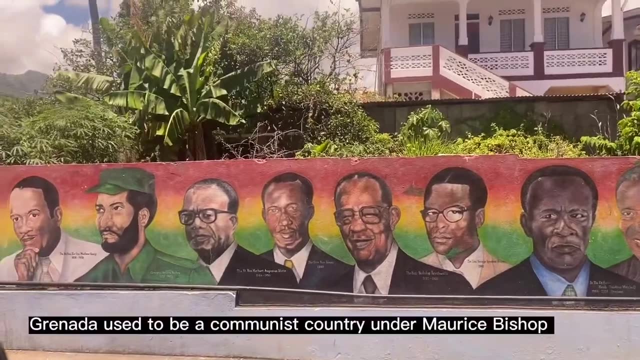 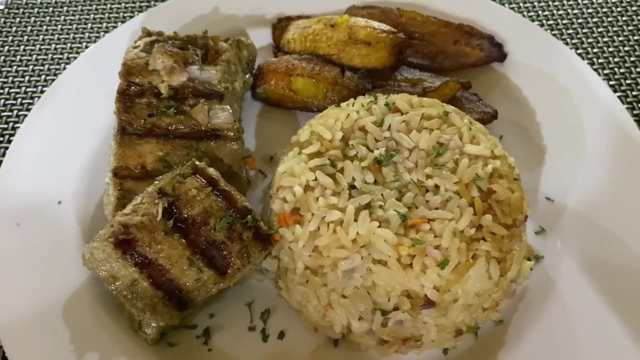 So doubles chickpeas: I like the butter, You like the butter one. Yes, Okay, It's good. Okay, Okay, You know it's very nice, beautiful, You know You can take a seat any time you want. 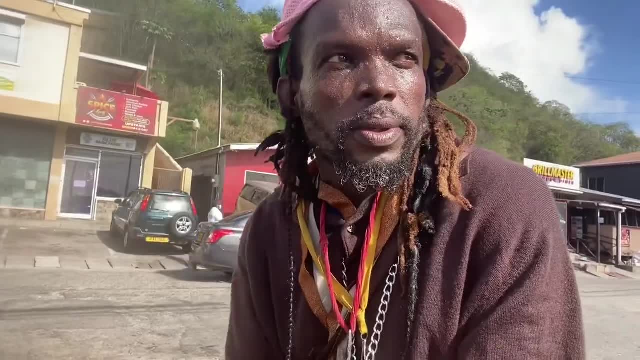 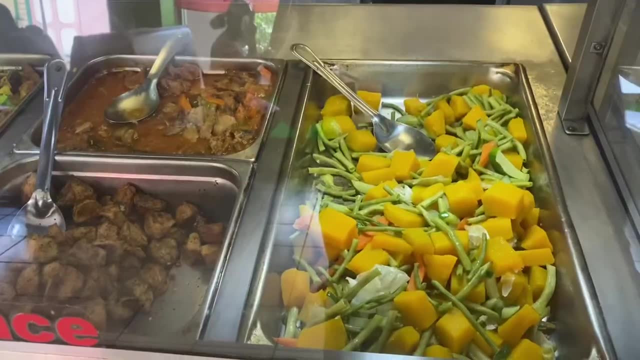 Very beautiful. Yeah, beautiful, But people tend to, Yeah, You know, enjoy the beautiful food. Yeah, The beautiful sea water. Yeah, You know that. I don't know what you're talking about. I don't know what you're talking about. 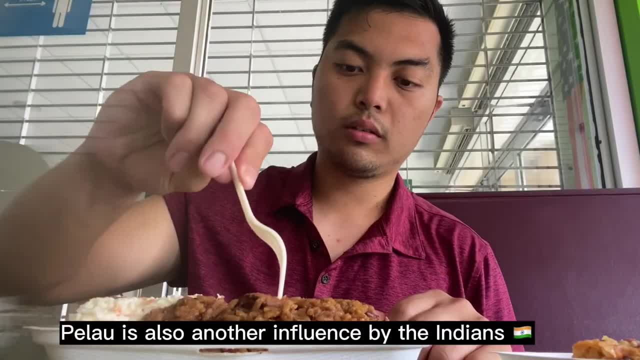 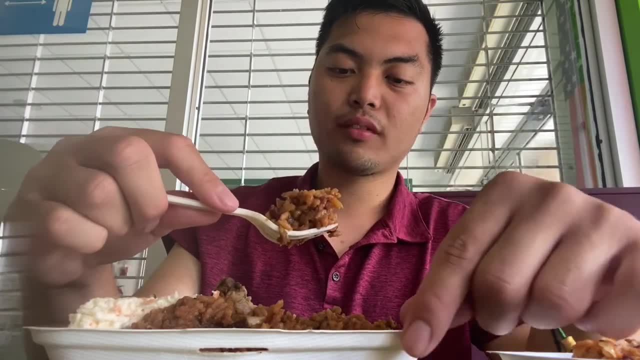 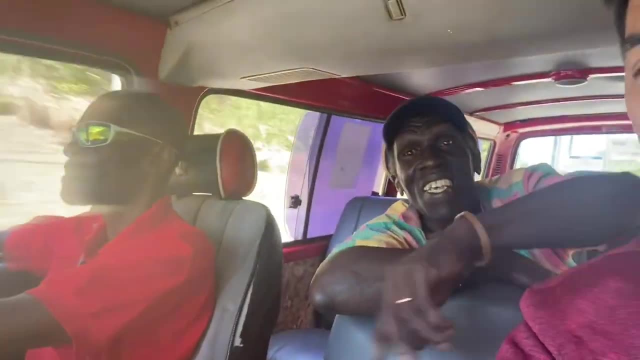 Okay, okay, Alright, hello, Hello. You can taste the beans. You can taste the beans and the rice and the grenadian flavor. and the grenadian flavor. I said the black sun, We have it. Sensimania, keep on burning, Don't you pander? Keep on brewing.